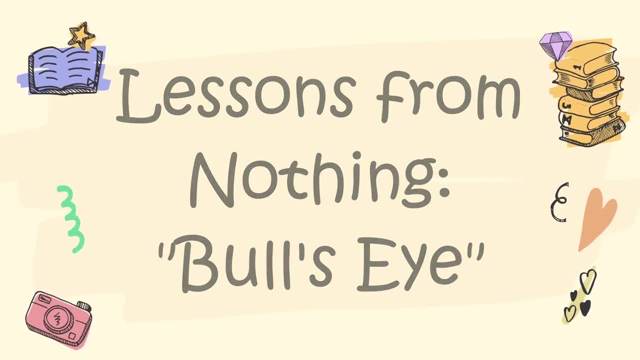 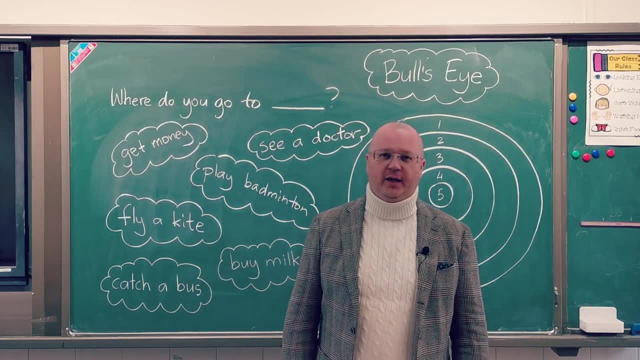 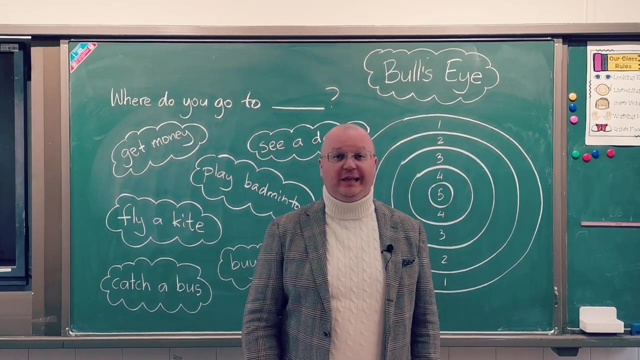 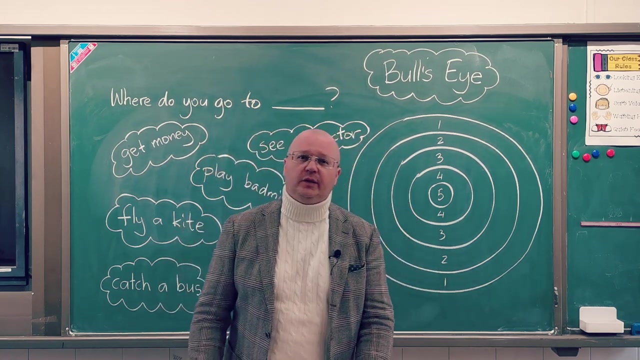 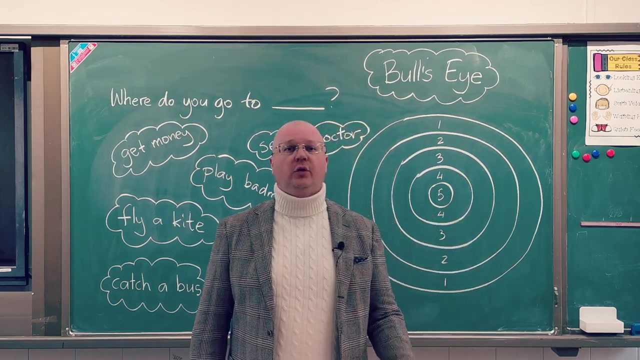 Hello guys, my name is Val and welcome back to my channel. In today's video I'm going to show you probably one of the oldest ESL games called Bull's Eye. It is a super simple game which is going to work for all levels. It's going to work in the kindergarten, it's going to work in grade. 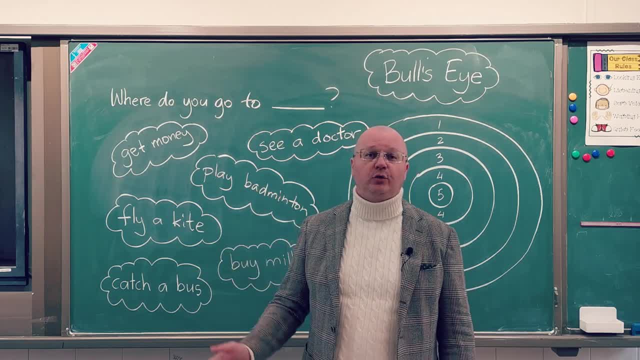 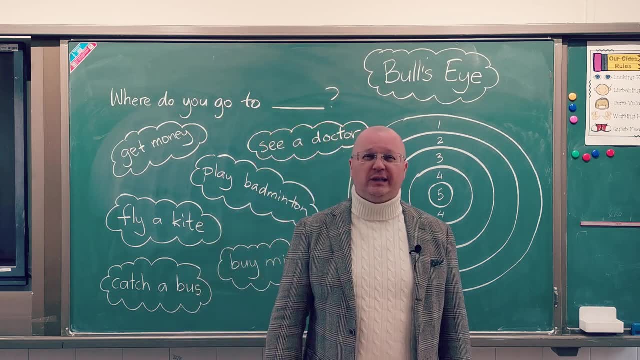 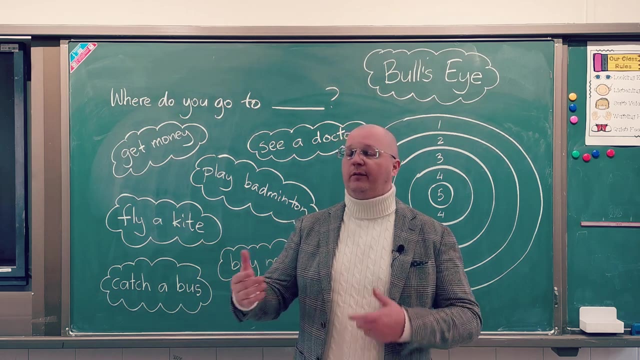 one to six. it's going to work in middle school, high school, even with adults. Everyone enjoys it very, very, very much. You probably know this game or you probably play some sort of version of this game already, but nevertheless, maybe there are a few people who do not know how to play it or want. 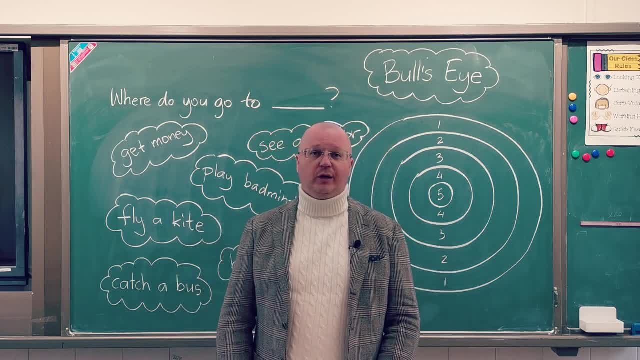 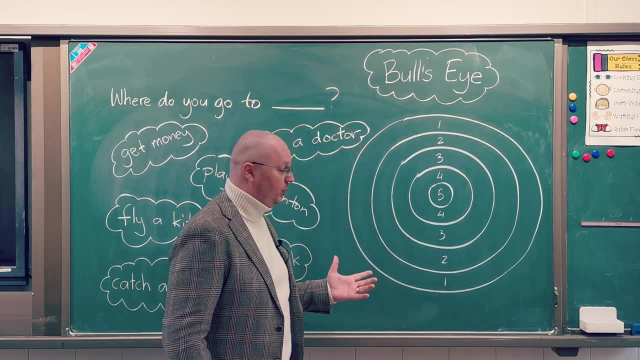 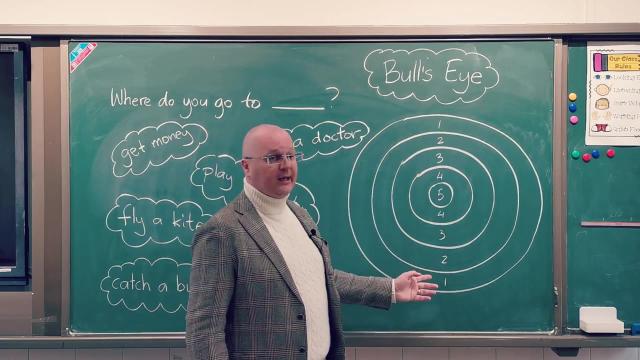 to see my version of it, So I am going to demonstrate how to do it. So, to prep this game, you literally need a piece of chalk and a blackboard or a whiteboard and a marker. You draw five concentric circles and, in my case, 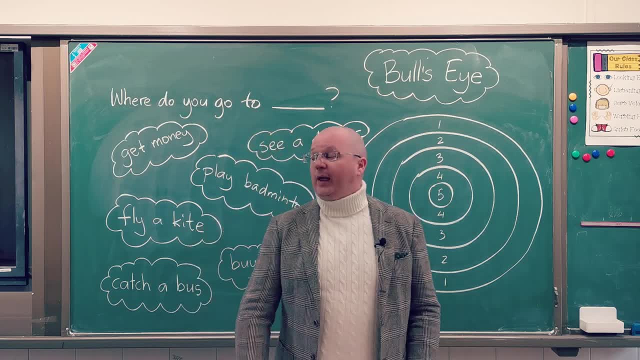 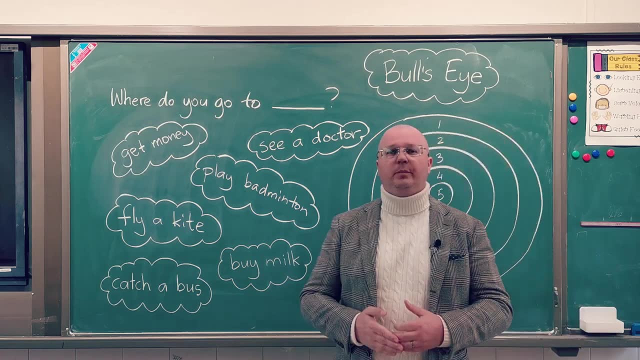 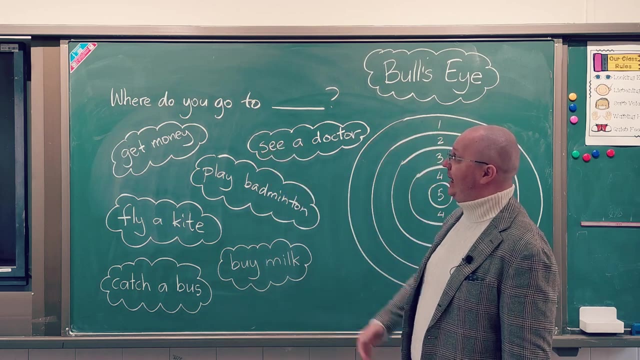 you mark them- one, two, three, four and five- And then you choose your target language. This could be a dialogue, this could be a passage, this could be a short report. It all depends on the level. So in my, in my case, it's the question: where do you go to, for example? 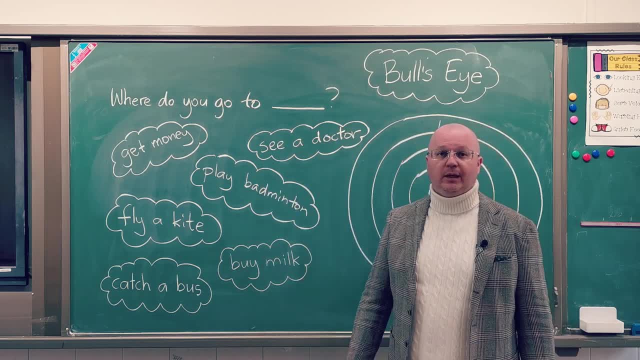 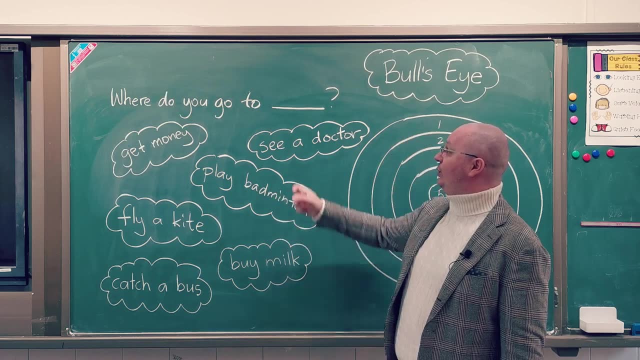 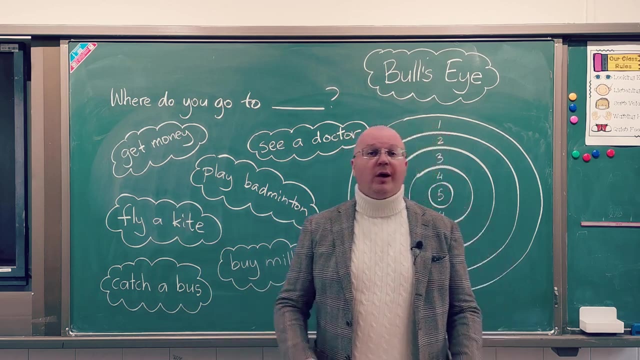 see a doctor, or where do you go to play badminton, and all that. And your students need to produce the target sentence, which is: I go to the hospital to see a doctor or I go to the bank to get money. So how do we play this game? 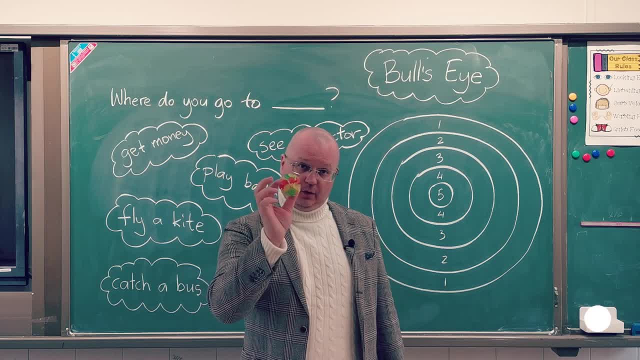 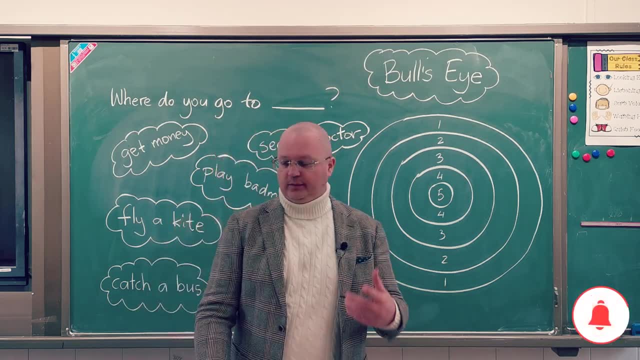 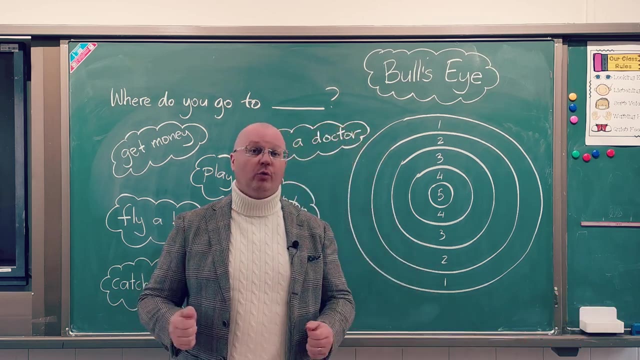 You will need either a sticky ball- It's a ball that sticks to the blackboard- This one doesn't stick very well, but doesn't really matter- Or a soft toy. That's all. That's all you need. And now let me show you how you play this game. 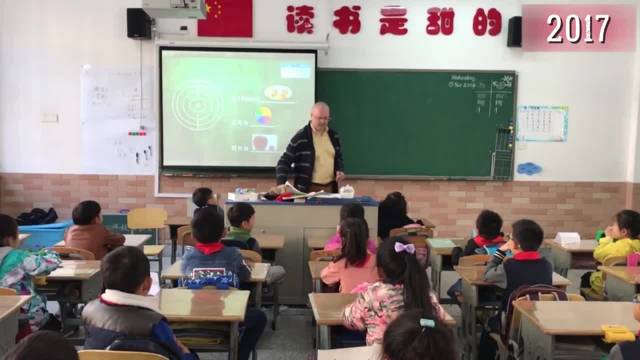 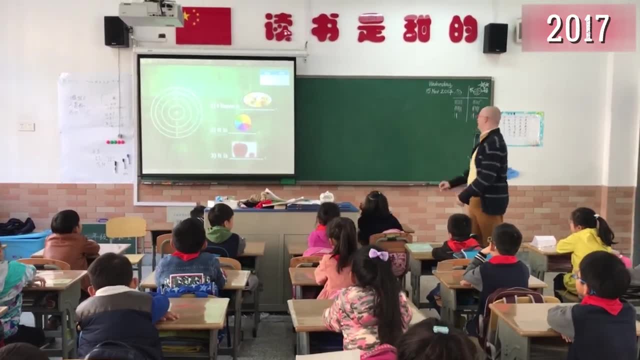 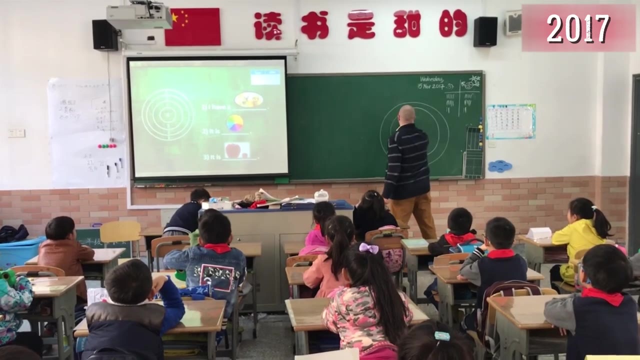 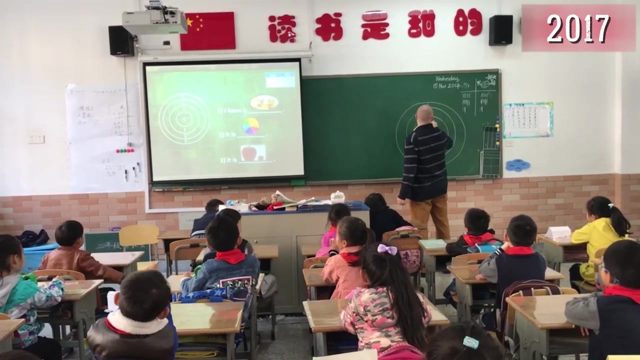 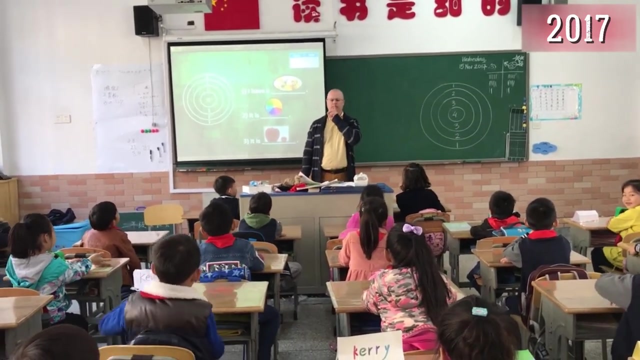 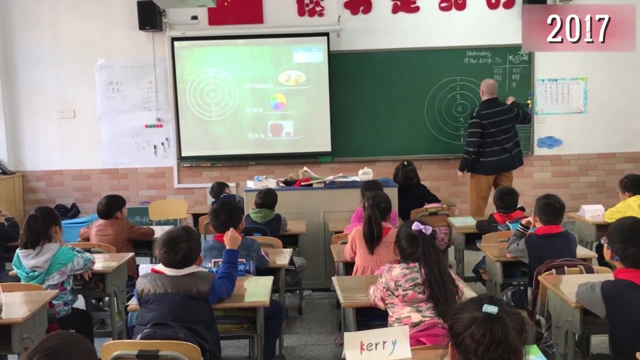 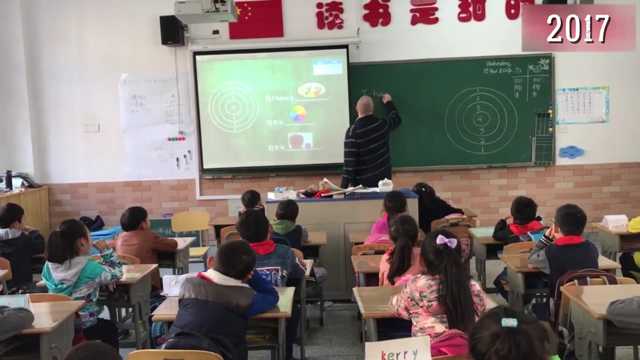 This is how we're gonna play. Alright, here we go. So this is one, two, three, four, Three, two, one. Thank you, Excellent. Look, we have three sentences. I have a. How much, how much, how much am I? 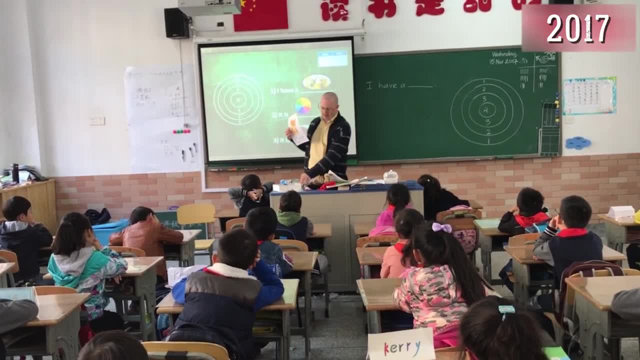 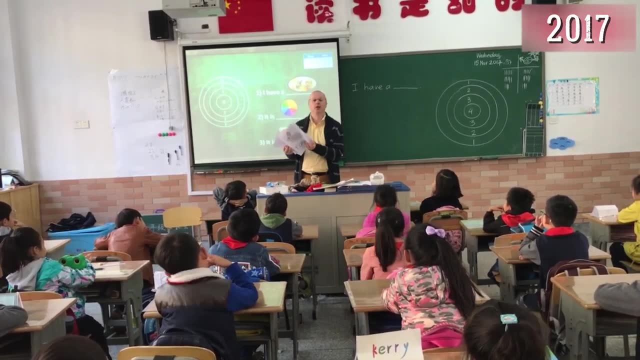 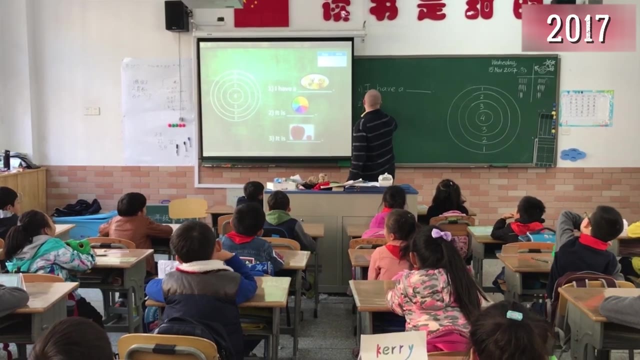 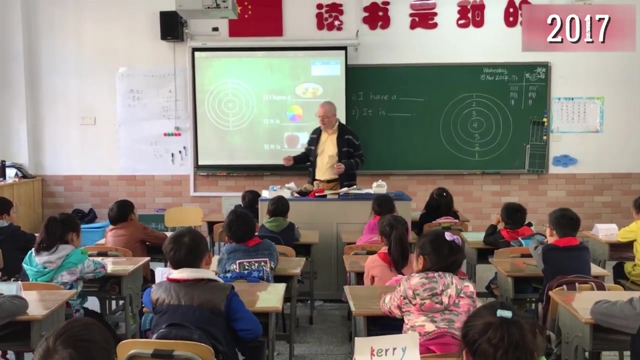 Animals. I have a cat, I have a hamster, I have a dog, I have a rabbit. Okay, Okay, Two It is. It is. What color is it? Yeah, What color is it? Is it blue? 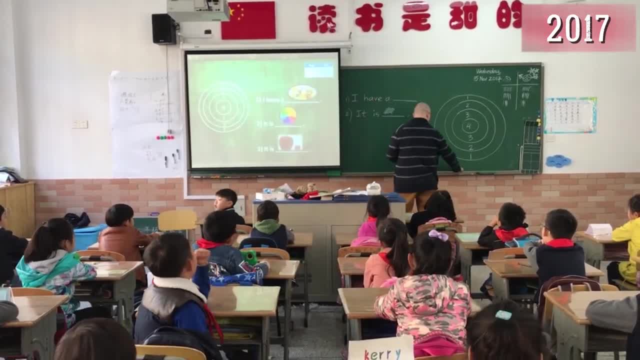 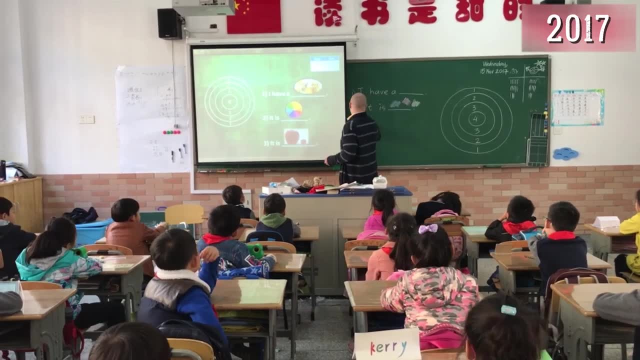 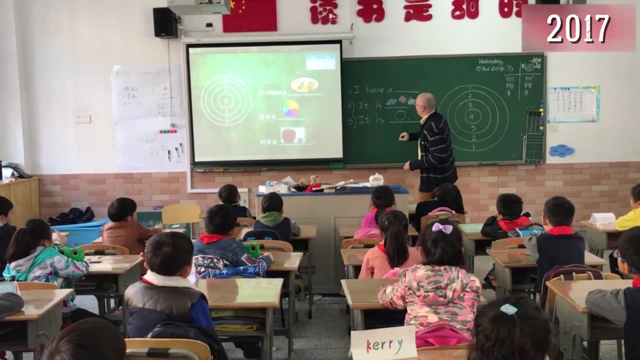 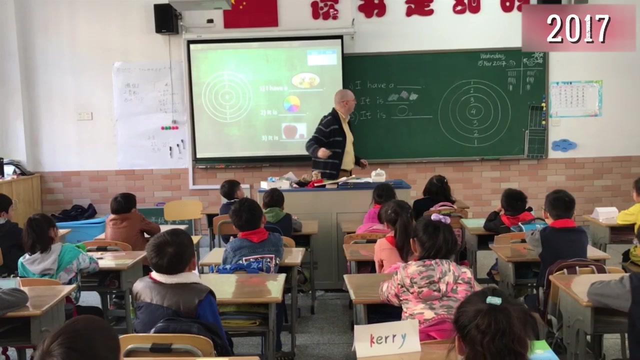 Is it blue? Is it orange? Yeah, Different colors, Okay, And three It is. It is Big or small. Big or small, Okay, All right. So this is how we play. Look, We are going to start here. 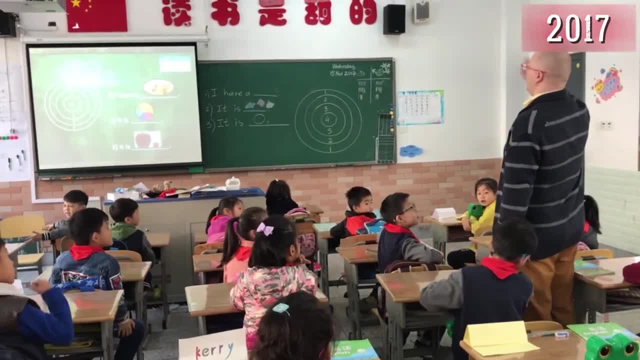 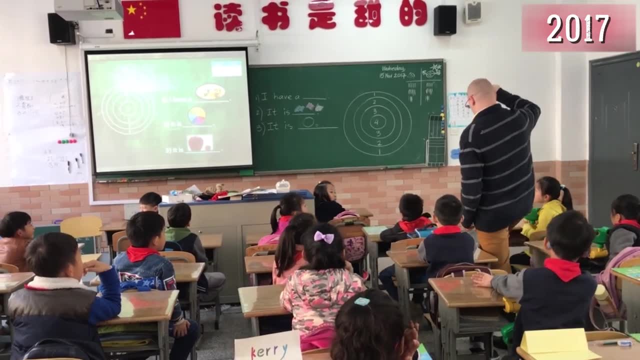 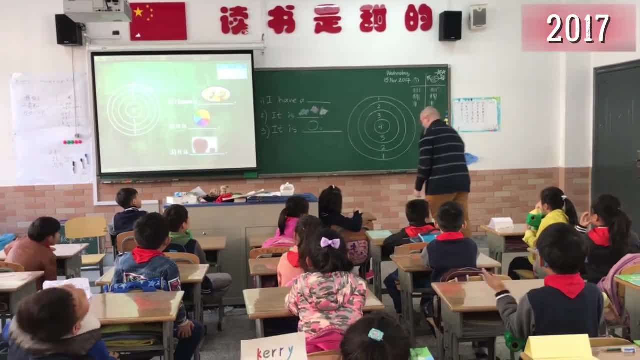 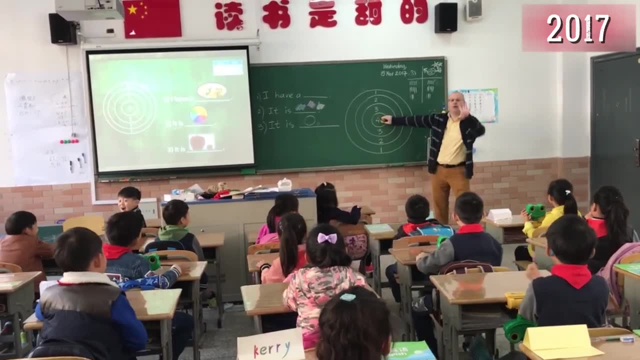 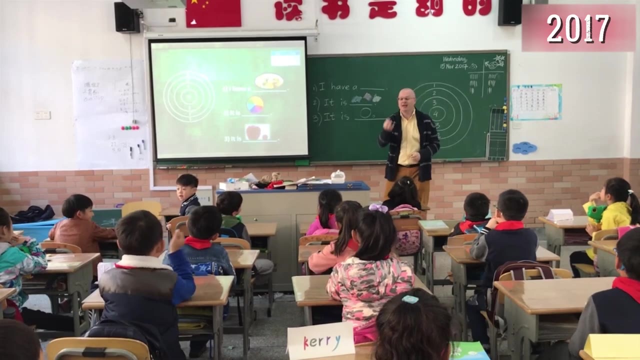 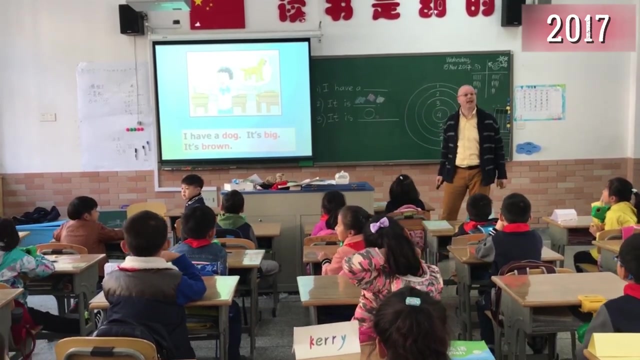 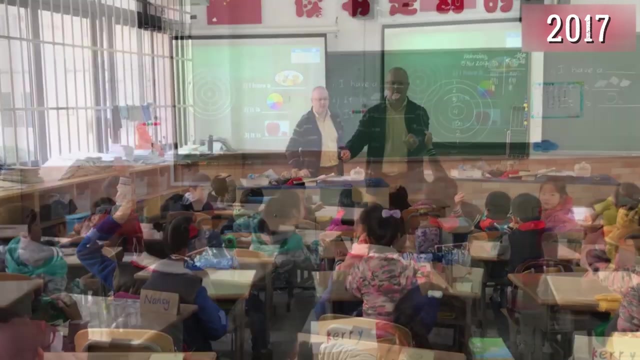 So I have three points Okay Here, Four points, Yeah, But you must say three sentences: Okay, Okay, You can look here. First you have to look at it, look and then say okay, okay, let's start easy, all right, all right, so rock paper scissors go. okay, ready.